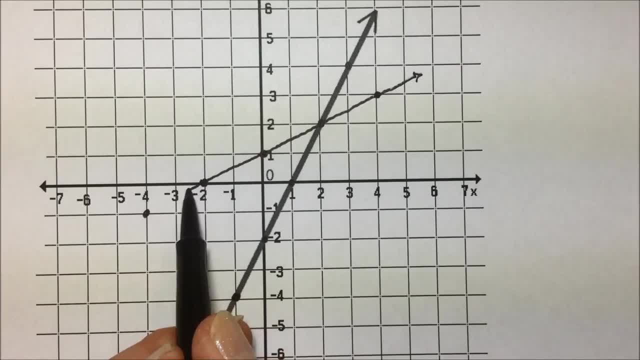 if I extend the line to connect those, we clearly can see that they are part of that. So here is the graph of our inverse: by just taking each one of our ordered pairs from the function and revolving it around, So we have the point of our original function. has the coordinate. 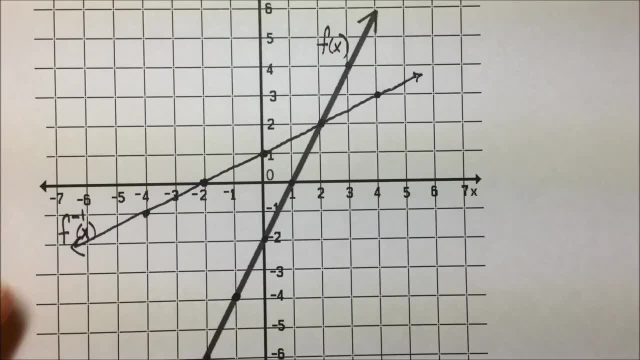 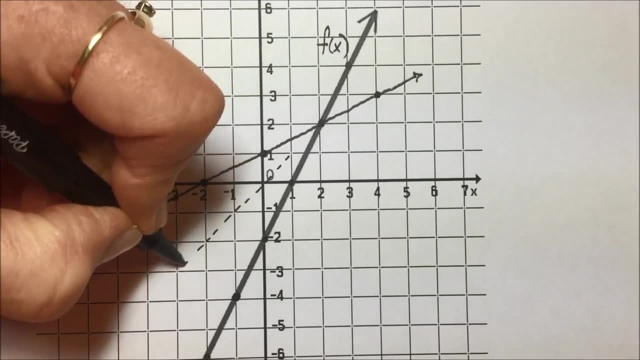 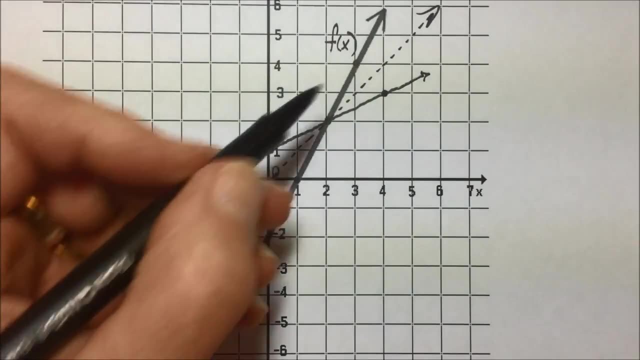 reversing them. The other technique, because we're reversing our x and y, is to reflect the points about the y equals x line And the y equals x line is at this 45 degree angle and you can see that here we have perpendicularly this point. If we reflect that about the line. 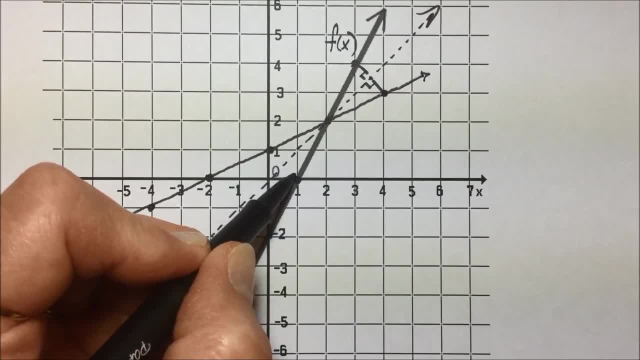 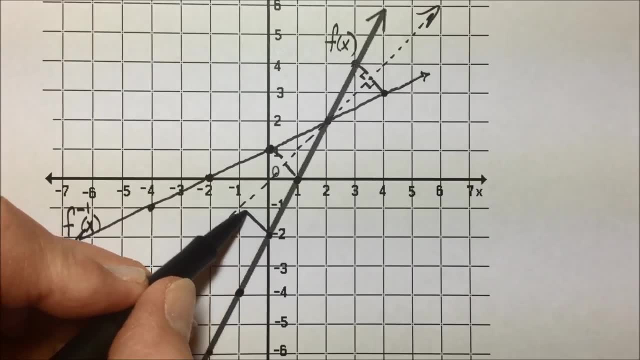 we would have the point Here on our original function, perpendicularly to our reflection line. we have a second point Likewise here, perpendicular this point on our function. if we reflect it through there, we have our point on our inverse function And we could. 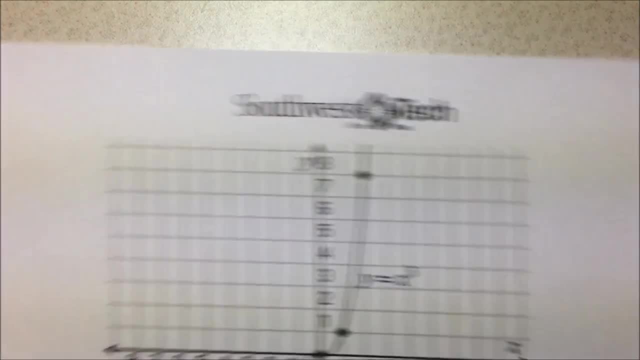 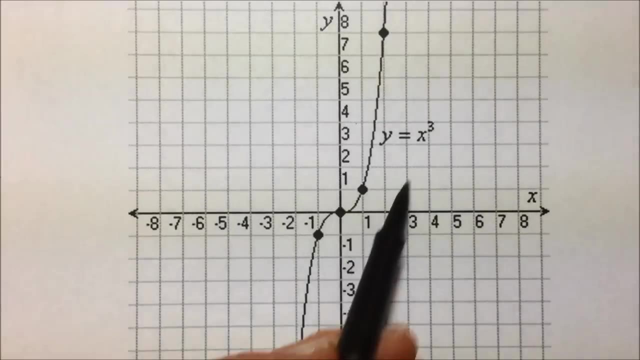 continue on for the graph. Here we have another function. It's a cubic function. It's given by y equals x to the third power. It passes the horizontal line test. Even though it flattens out here, it's still moving along and would only if we ran the horizontal line test intersecting once, Because it's 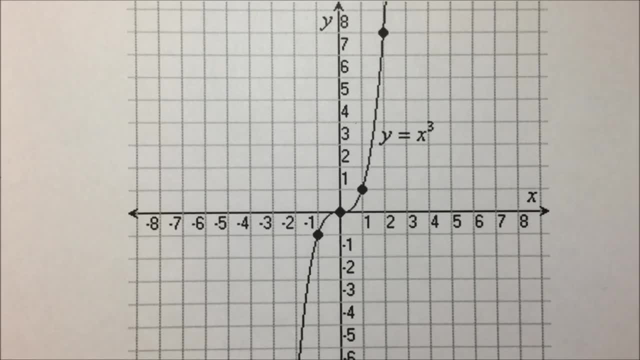 passing the horizontal line test is proof that this is a one-to-one function and that it does have an inverse. You have again two choices for graphing an inverse of a function: either point or inverse. And so we're going to draw that, We're going to add an inverse measure to this line by: 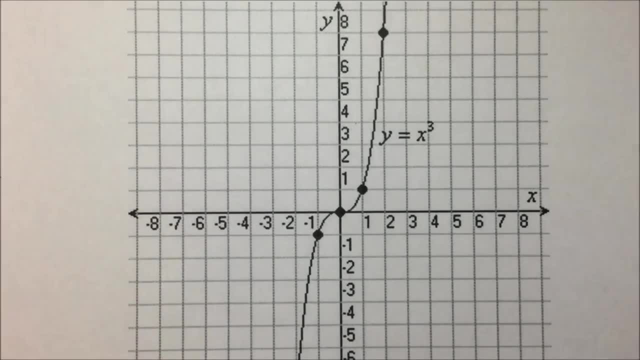 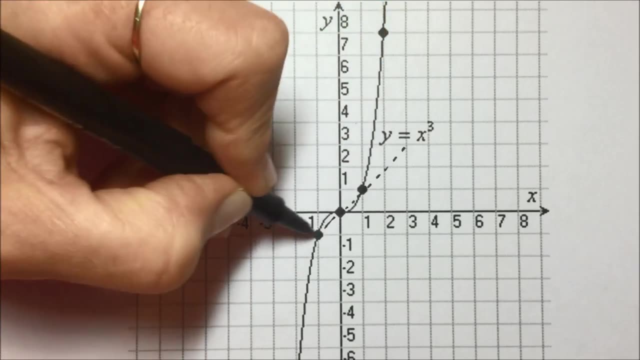 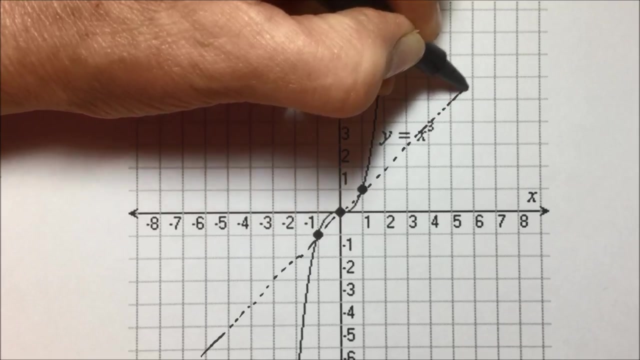 tissue, So that we have an inverse of both cases. The first concern is that let's say we have a center point And let's say we want to take x to the first coefficient in our sum And let's convey that the marked value is point to cell to one. It'llcellicise that. 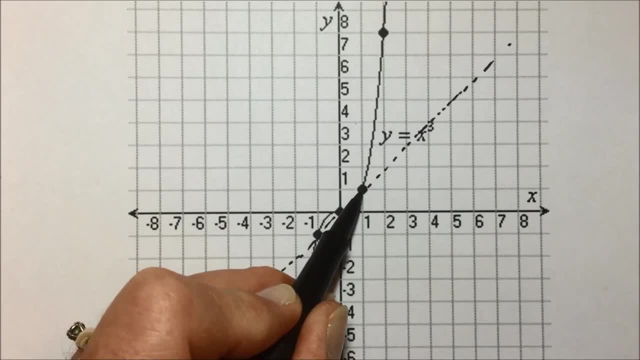 to z. Let's Q II is curving here. below will actually be curving above. What's curving above will actually be curving below. So here, if I make this a little heavier, you can see the beginning of our inverse function. We can either turn this point around as part of our original function.